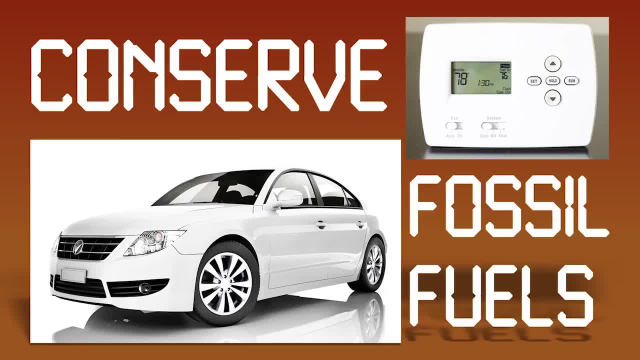 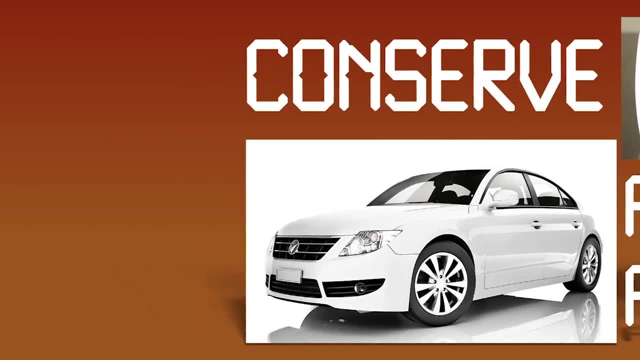 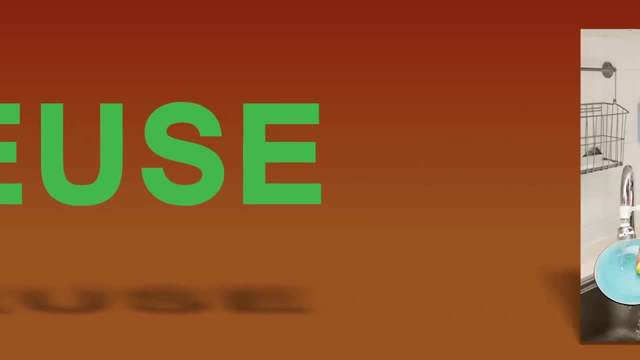 can reduce the amount of natural resources they use. Reducing the amount of fuel used to heat homes or choosing to drive more fuel efficient cars will help conserve natural resources. Reusing materials also saves natural resources. There are many products that can be reused. You can use washable dishes instead of disposable dishes. Think about the amount. 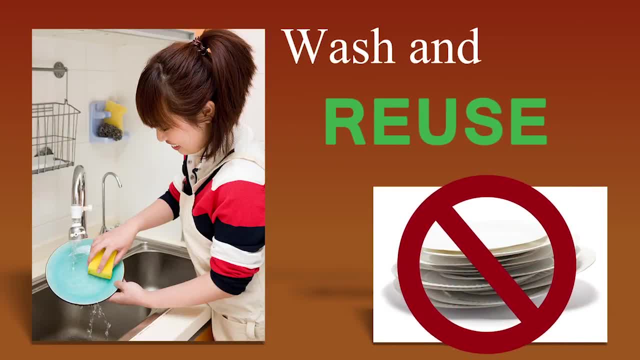 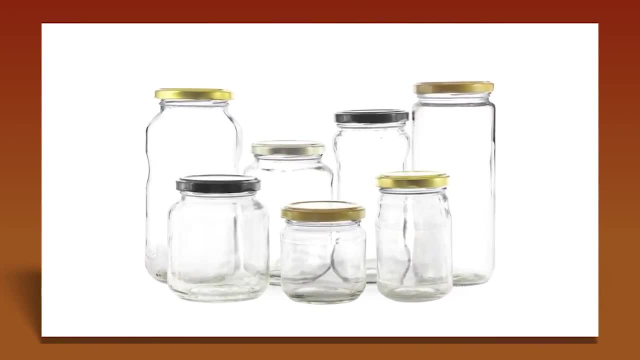 of garbage that piles up in landfills from paper and foam tableware. Using washable dishes cuts down on waste. Look in the kitchen and you will find numerous containers that, when empty, can be reused instead of being thrown away. Empty pasta sauce jars can be used as 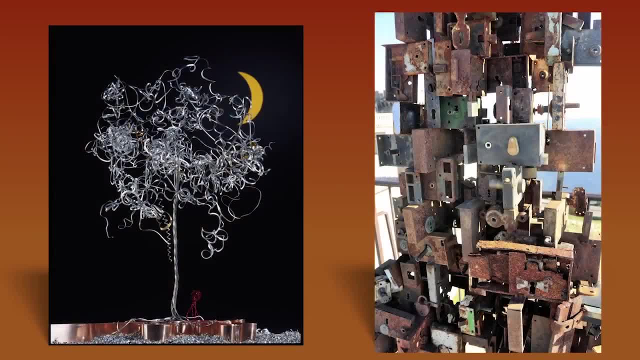 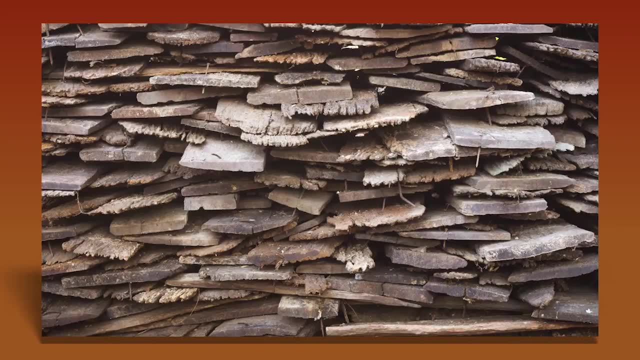 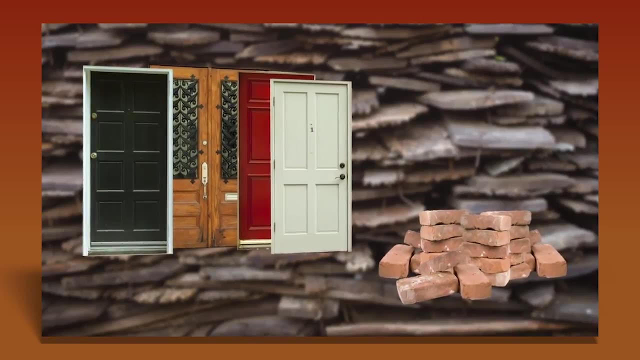 storage for nails and screws in the garage. Modern artists have made many amazing and unique sculptures for materials they found to be reusable. One idea that's gained popularity is reselling building materials. When a house or building is torn down, a crew will remove. 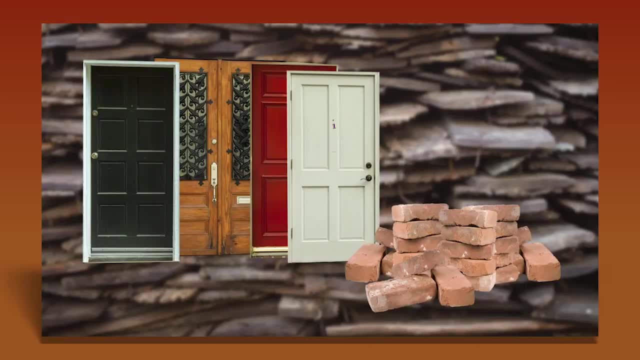 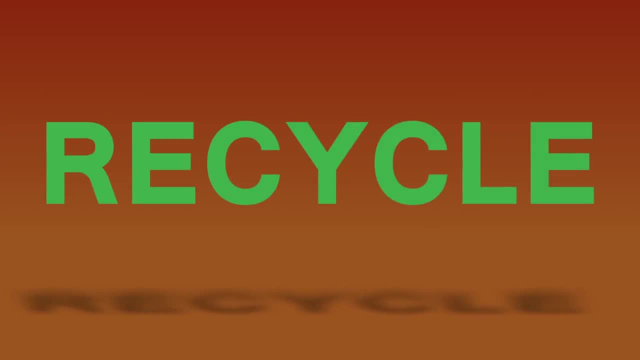 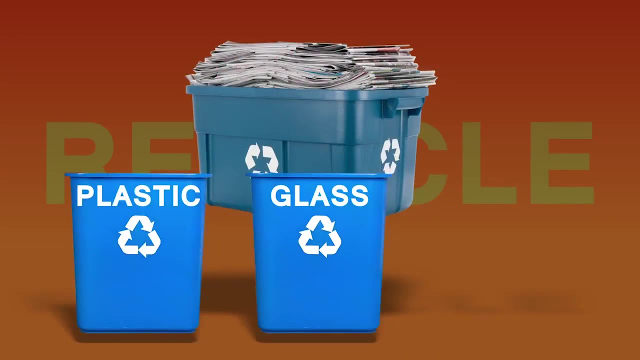 all usable materials. These items are sold to contractors or homeowners to be reused in new homes. People can also save resources by recycling materials that can be reused in new ways. You can separate your trash for recycling and take paper products, plastic, glass and. 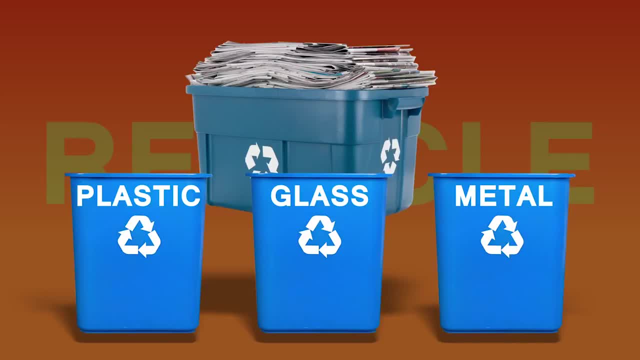 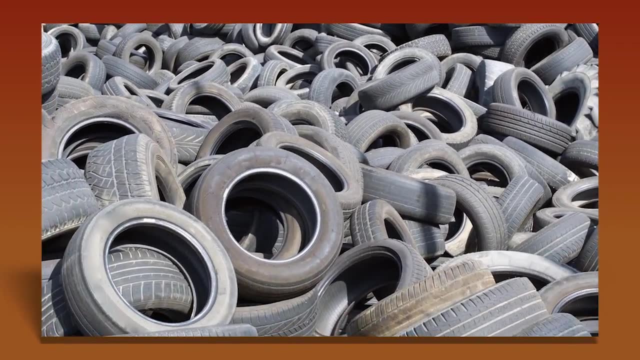 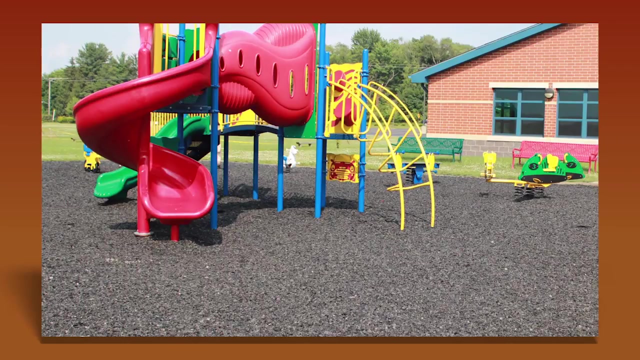 metal cans to recycling centers. These products can be recycled and reused instead of piling up in landfills. Many new playgrounds are covered with shredded rubber mulch that has been recycled from tires. This recycled rubber protects children from being injured while keeping waste out of landfills. 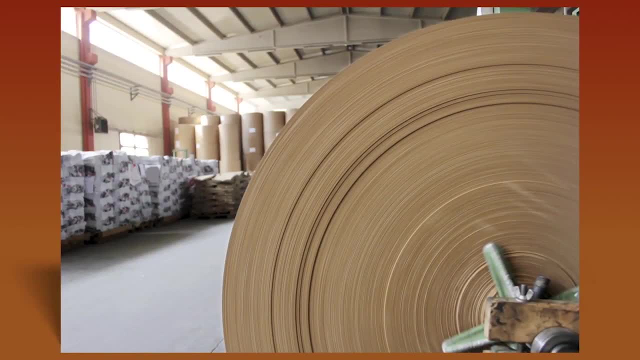 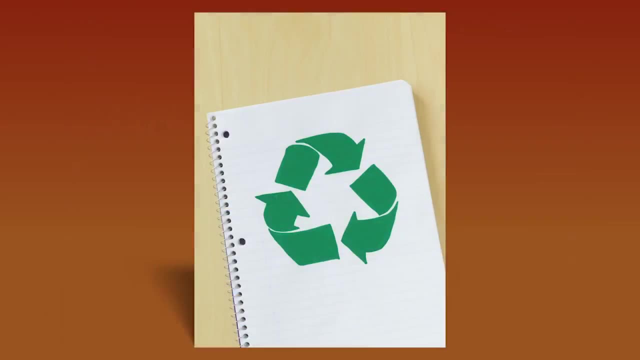 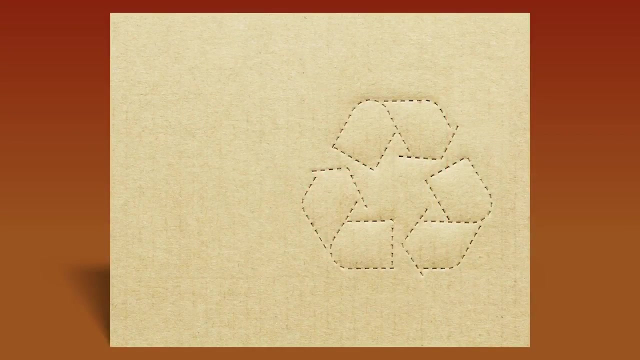 Recycled paper is washed and combined with other materials to create a special mixture. This mixture is spread using large rollers into thin sheets. Once dried, these sheets are cut and used for new, clean pieces of paper. Recycled paper can also be turned into. 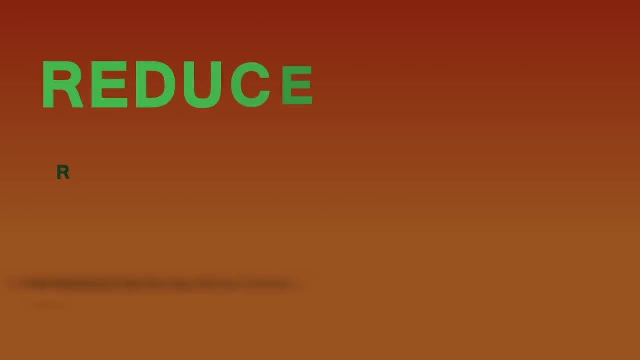 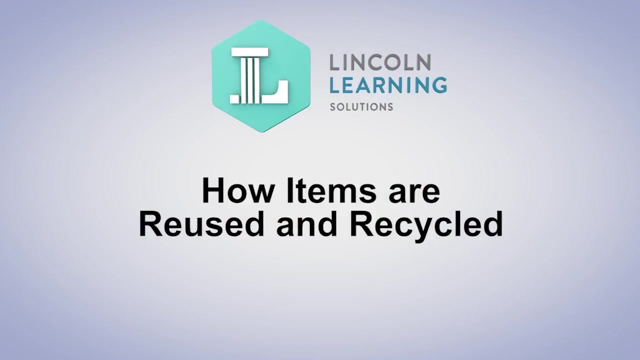 cardboard or newsprint. Reducing, reusing and recycling waste keeps garbage out of landfills and helps to protect the environment. For more information, visit wwwfemagov.